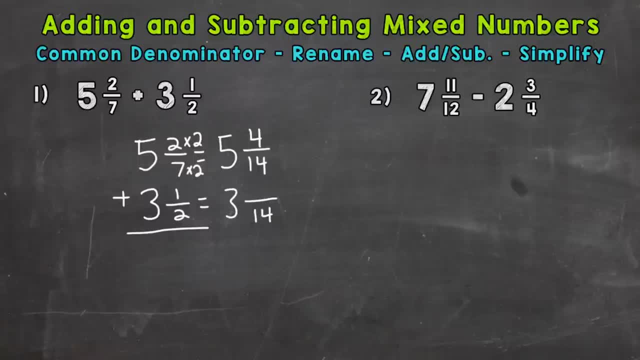 So 2 sevenths is equivalent to 4 fourteenths. So we renamed with that common denominator, least common denominator of 14. So let's do it to the half here. We know that 2 times 7 is 14. So do the same exact thing to the top to keep it equivalent. 1 times 7 is 7. And this is addition. So now once we have that common denominator and we renamed, we're able to add or subtract. 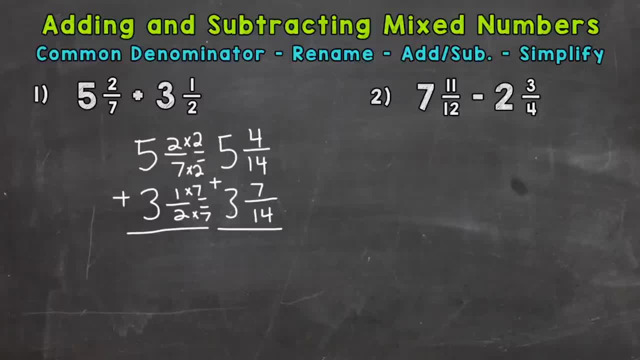 So let's add our fractions first. 4 plus 7 is 11. And this is fourteenths. And then we add our whole numbers. So 5 plus 3 is 8. So once you get to that point, check to see if you can simplify the fractional part. So do we have any common factors between the 11 and 14? Well the only common factor is 1, so this is in simplest form. Our final answer is 8 and 11 fourteenths. 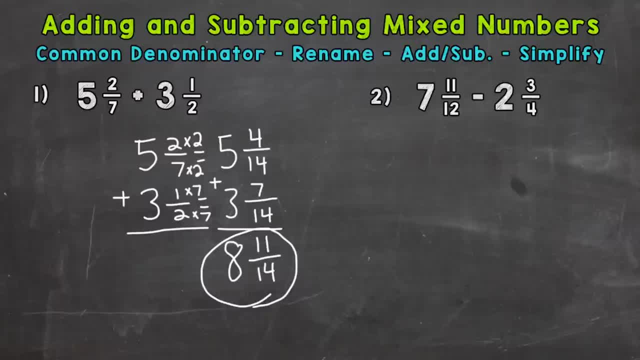 Let's move to number 2 where we have subtraction. And subtraction is the same exact thing that we just did, but instead of adding, we're going to subtract. 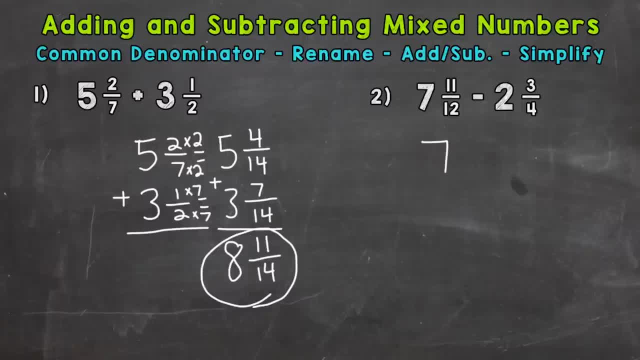 So let's line up vertically up and down. So 7 and 11 twelfths minus 2 and 3 fourths. So do we have a common denominator between our two fractions? Are we able to subtract right away? No. So we need to find a common denominator. And the least common denominator between a 12 and a 4 is going to be 12. So let's rename. 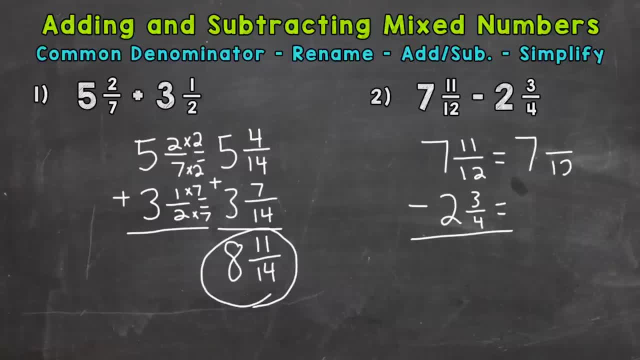 So we have 7 and how many twelfths? And 2 and how many twelfths? Well, 7 and 11 twelfths already has a denominator of 12, so we don't need to rename. 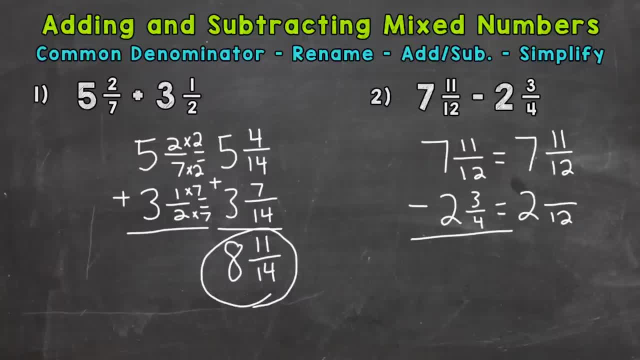 So let's transfer our 11 over. Now we do need to rename the 3 fourths. So we know 4 times 3 is 12. Do the same thing to the top to get an equivalent fraction here. So 3 times 3 is 9. 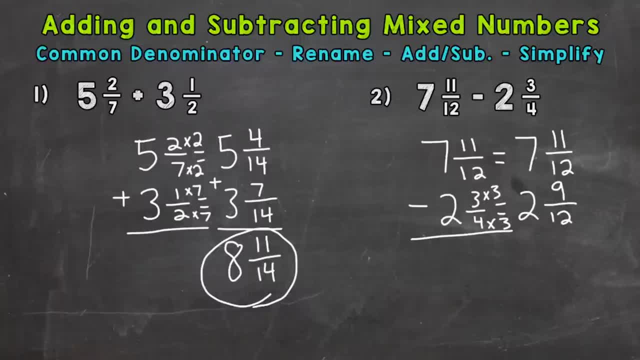 So 3 fourths is equivalent to 9 twelfths.